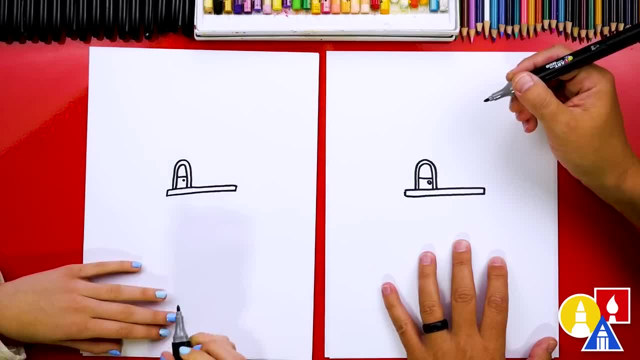 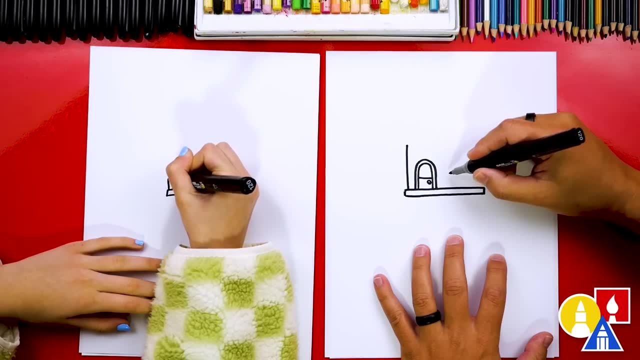 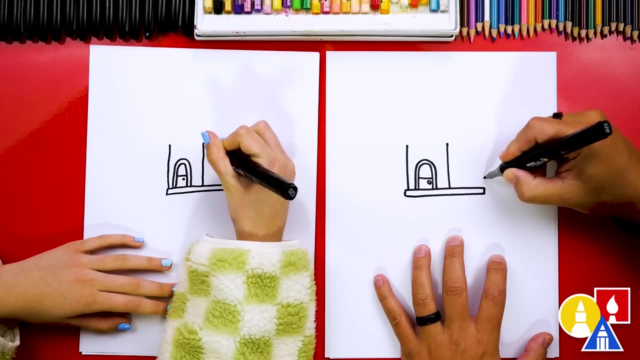 We have to add a doorknob, a little circle, there. Now let's draw the rest of our tree house. We can draw one line that comes up here and Then let's draw another line that comes up to match right next to it, And then let's draw another line over here to match also. 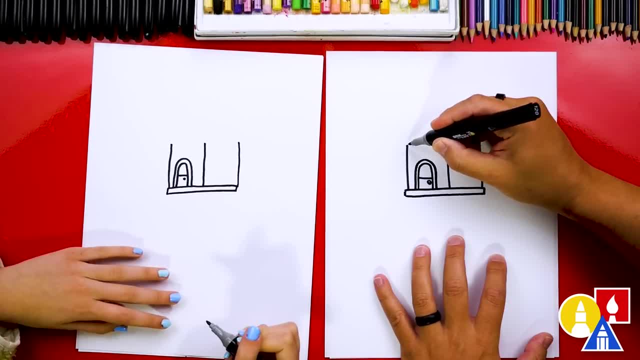 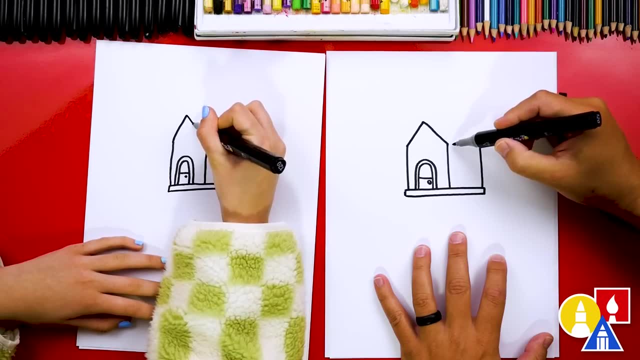 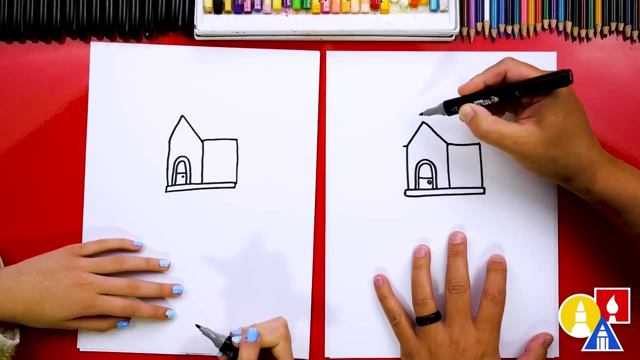 Yes, okay, now let's add a little upside-down V right here to connect these two lines. Then we're gonna draw a straight line across to connect to the last one, and then let's add a little Roof on top. We're gonna draw a short line here. 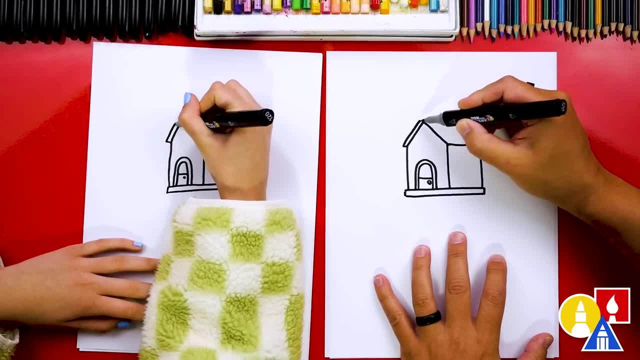 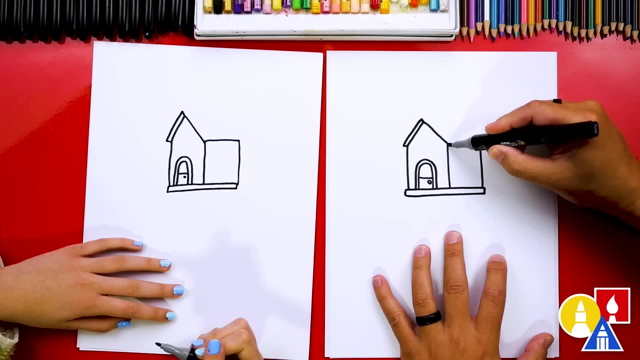 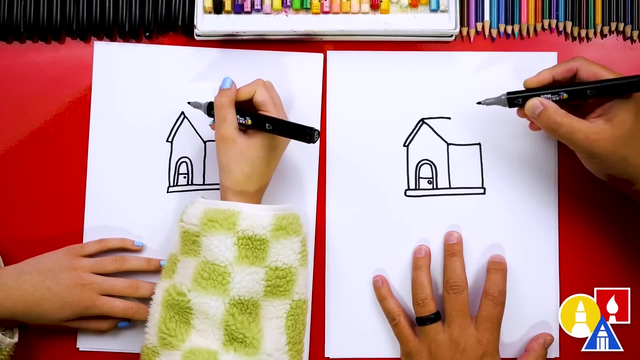 then we're gonna come up and Right here let's actually connect so it looks more 3d. Then we're gonna draw a line, We're gonna pretend to copy this line and we're gonna paste it up here. So we want the same length line up here at the top. 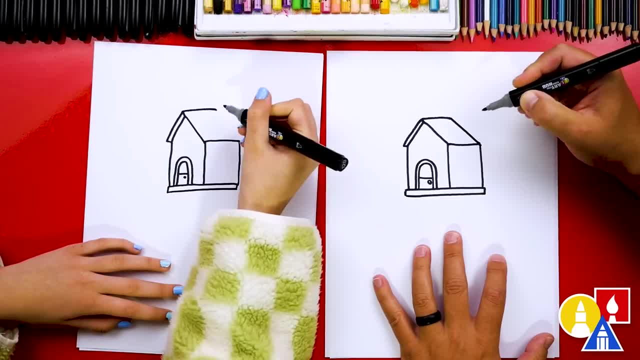 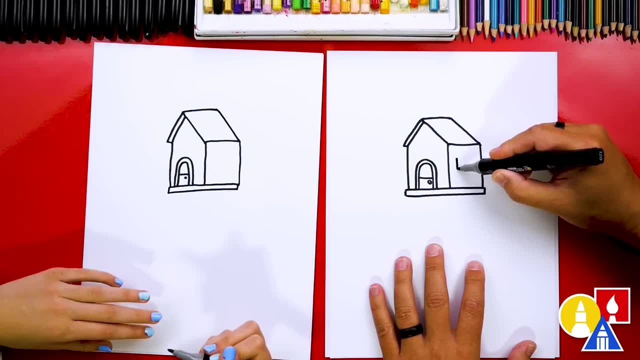 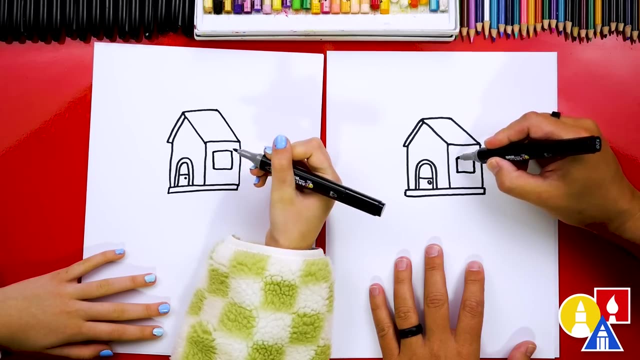 And then we're gonna draw a diagonal line down to connect. There's our roof. now let's add more details to our tree house. we can add a little window right here. I'm gonna draw a rectangle shape And we could also add shutters. and also the fun thing with art is you can add all kinds of different decorations. 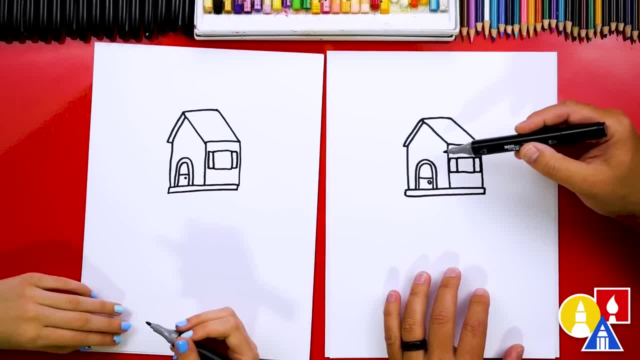 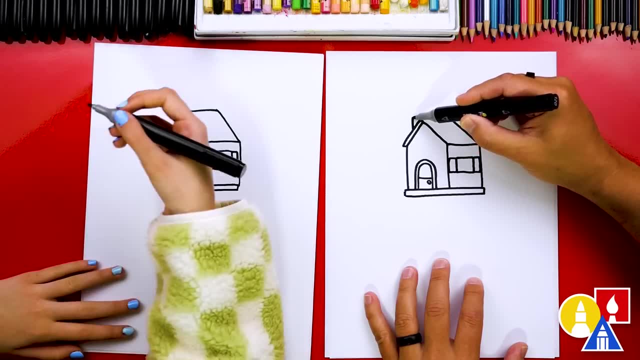 To your drawing so you could add designs to your tree house, You could add more windows, You could even add a chimney. Oh, that would be fun. Oh yeah, little chimney. Okay, let's do that. Let's add an upside-down or just a rectangle shape. 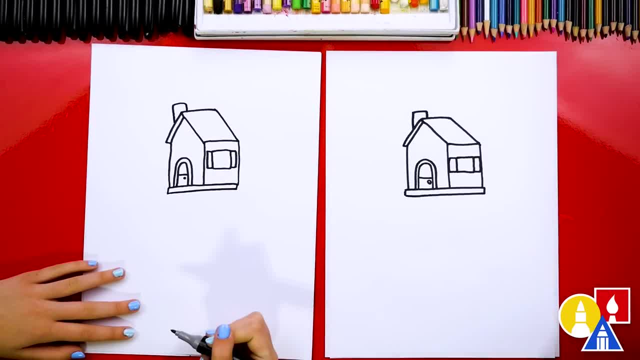 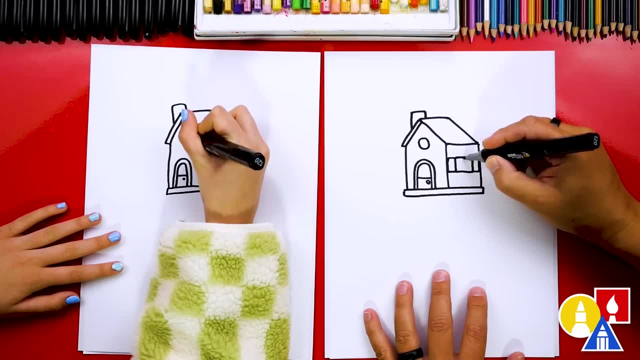 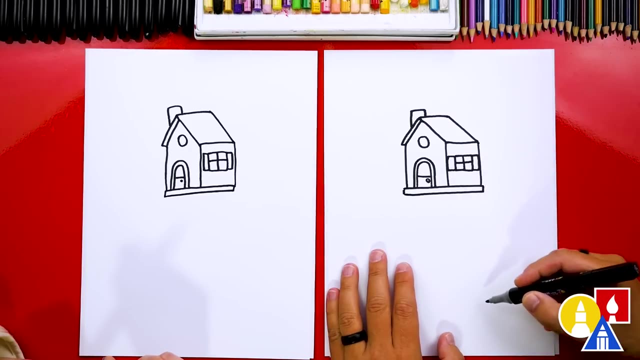 I was gonna say: upside-down you. There we go. That's a simple little oh, and we could also add a little circle here for the top one. Oh, oh, I'm gonna add more details a little, plus sign in the window: Now let's draw the ladder that's gonna get us up to our tree house. We're gonna draw a. 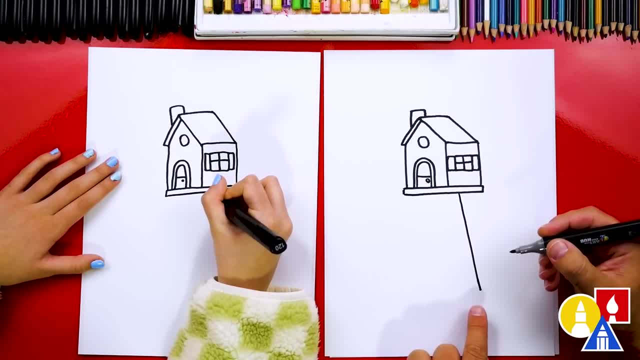 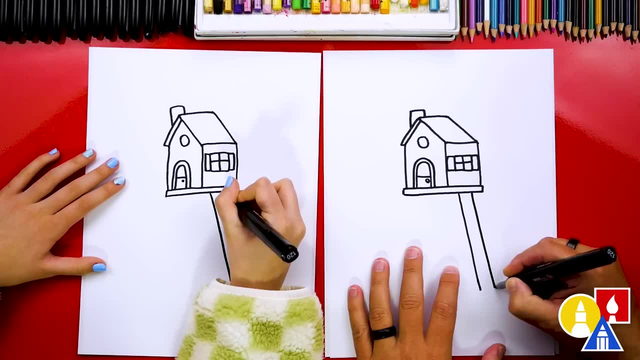 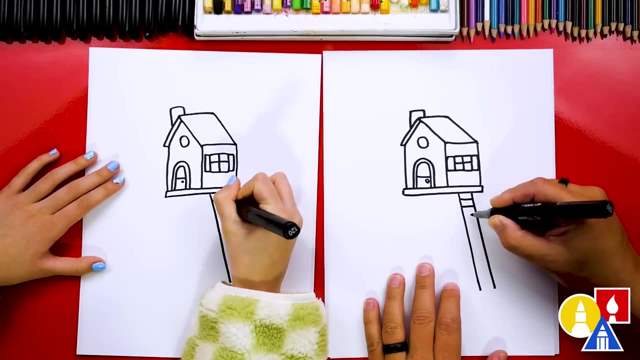 diagonal line that comes down and we can just pick wherever we want to stop. this will be the ground or the bottom of the tree- and Then we can draw another line right next to it For the other side of the ladder, and then let's draw the steps. So we're gonna draw lines going this way. 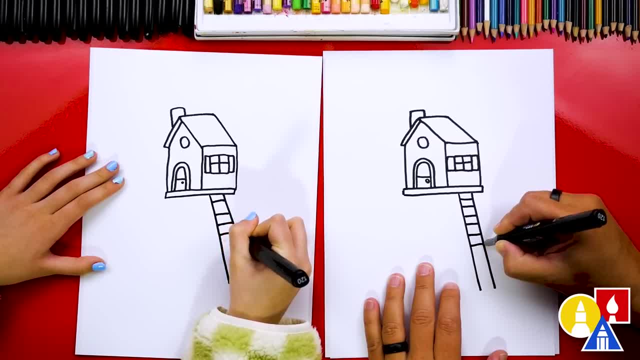 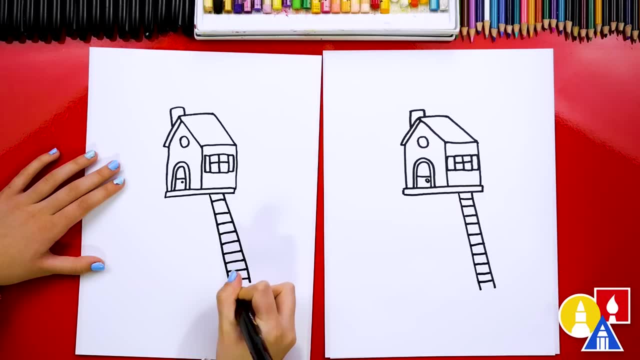 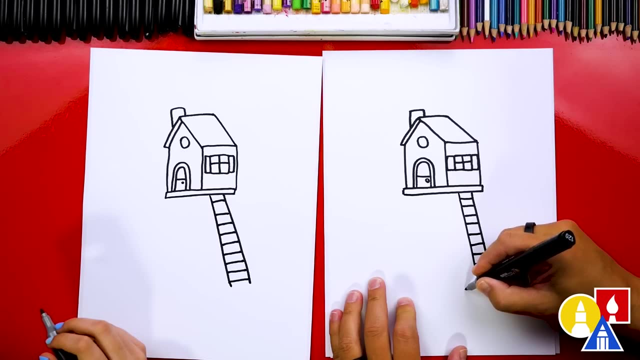 And we want to try to evenly space them all the way down until we get to the ground. Yes, Good job. Okay, Now we're ready to add the tree. Let's start here and we're gonna draw a curve. We'll start here. I'm gonna draw curving up like this, and you can really change this any way you want. 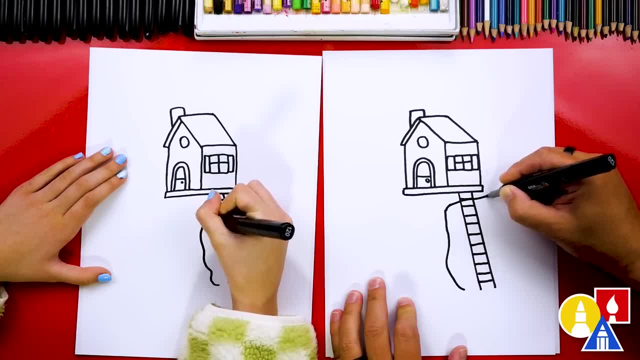 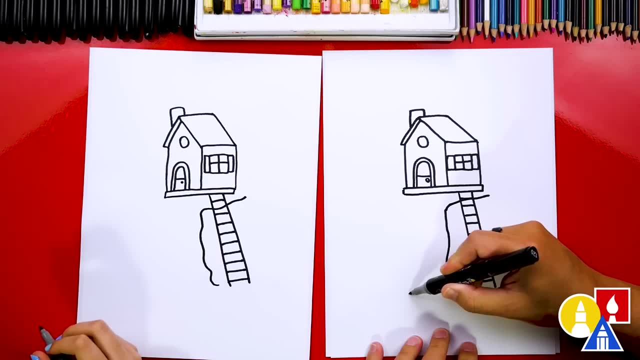 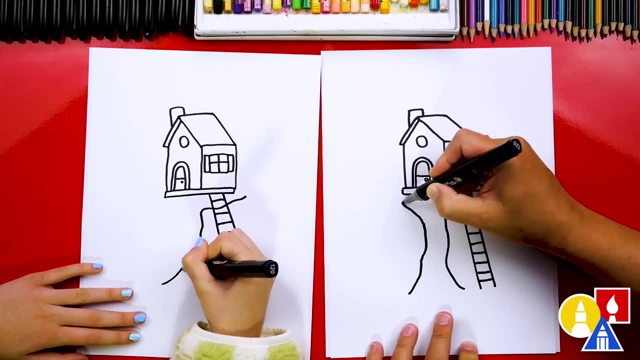 I'm gonna curve here and even go underneath the tree and the ladder, or sorry, The house and the ladder. Okay, Now let's draw the other side of our tree. We're gonna start here and curve up so we get kind of close To the other curve that we were drawing, and then I'm gonna come out this way: 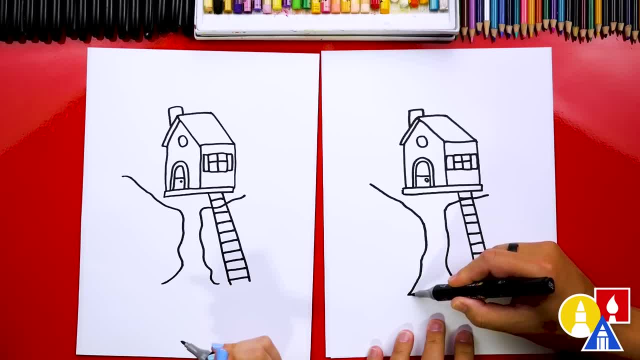 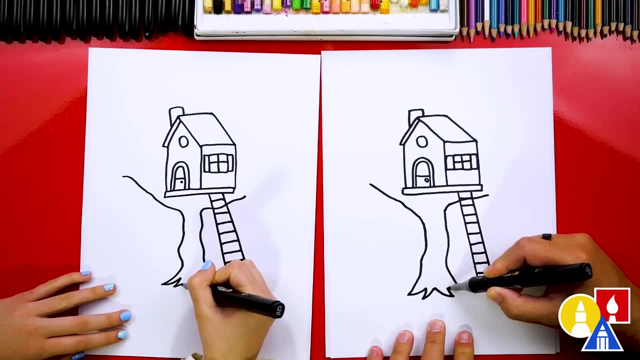 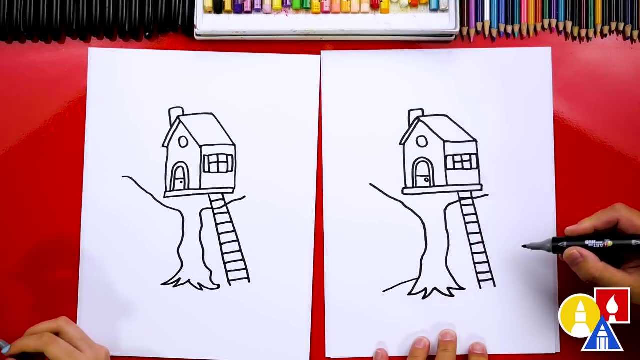 Yes, good job, now we can add the roots down here. I'm gonna draw a zigzag line For two roots, maybe going this way, and then a zigzag line for two roots going the other way. Then we can also draw the ground. I'm gonna draw a curve coming out this way and 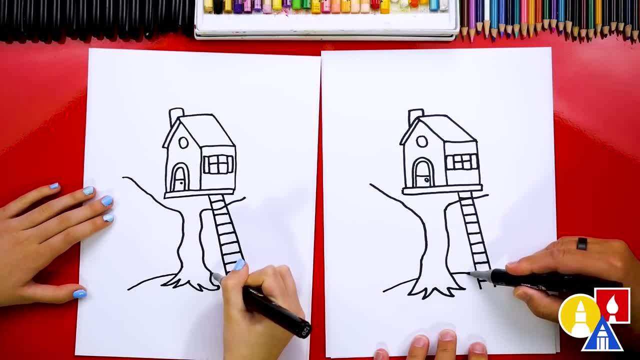 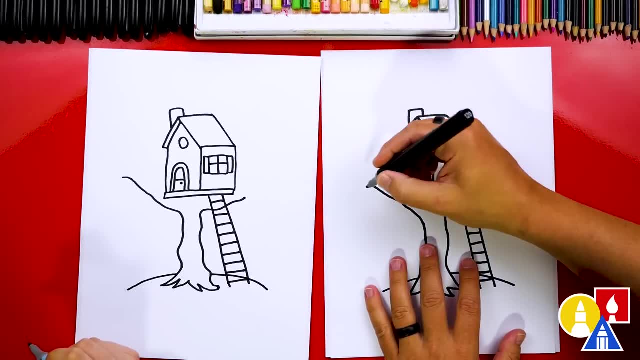 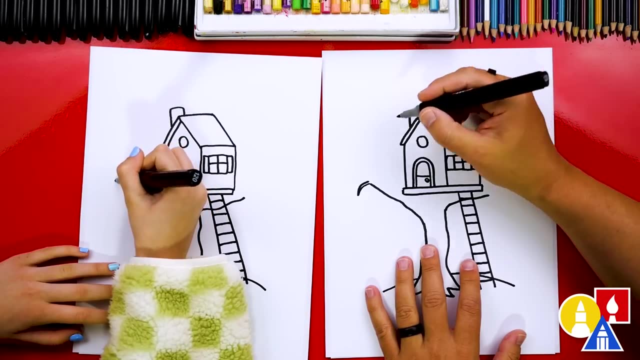 We'll draw or imagine that curve going behind the tree and coming out this way: Yeah, okay, now let's draw the branches for a tree. I'm gonna start over here and we can curve out and then back in. Let's draw another curve out and back in and kind of drawing these sharp. 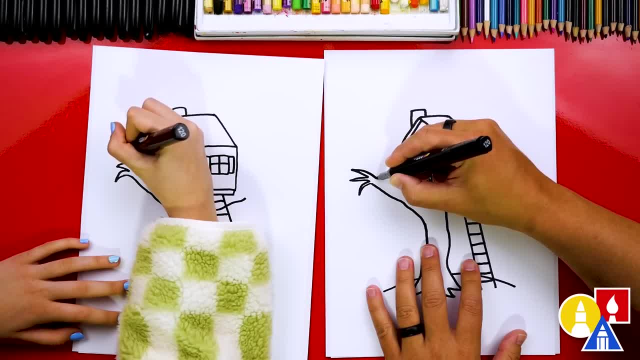 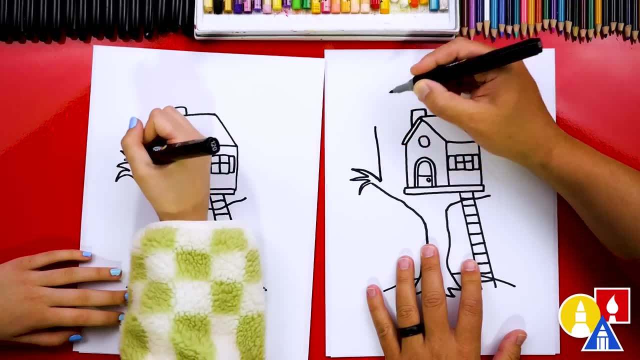 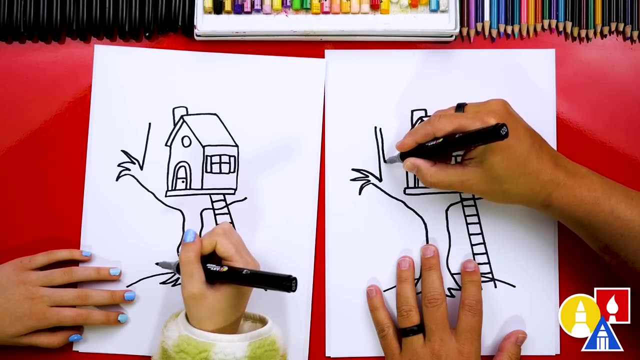 And then I'm gonna do another one that comes out and back in. so we got three Little branches coming off of this bigger branch and then we can draw. let's draw a branch coming straight up from this bigger branch. I'm gonna leave a little space right here and we're gonna draw the other side of that branch coming down. 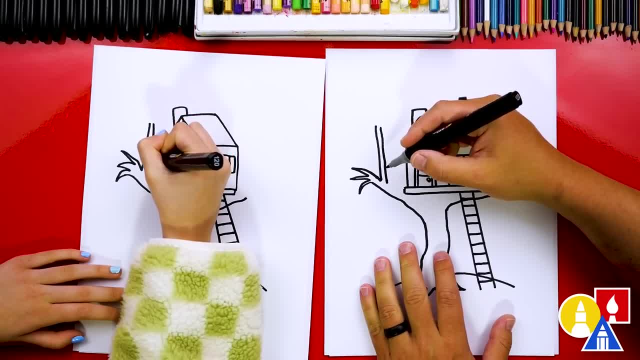 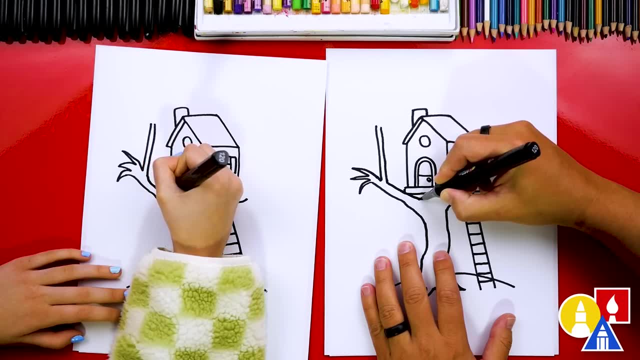 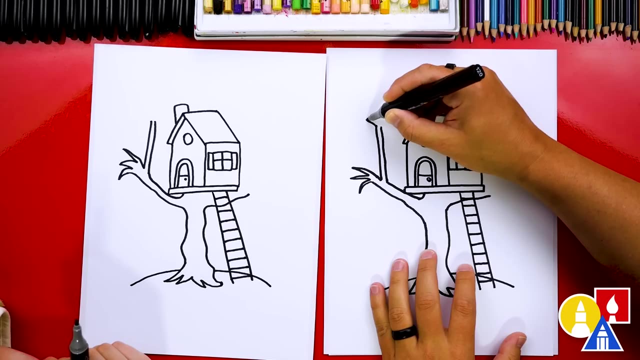 To where this bigger branch is coming out. then we can draw it coming underneath the treehouse and leave the branch open. And now we go to another side and laid the huge branch underneath. Okay, I'm going to, of course, make this part recognize. What we did here was I drew a system. 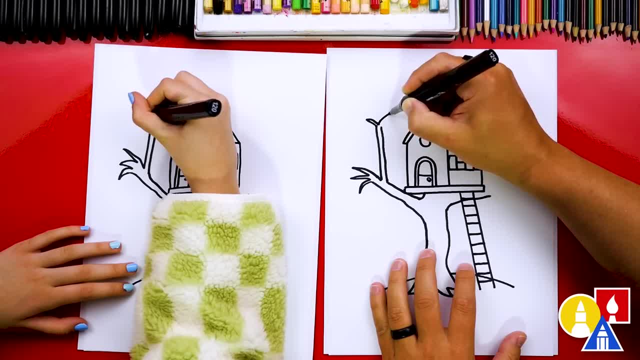 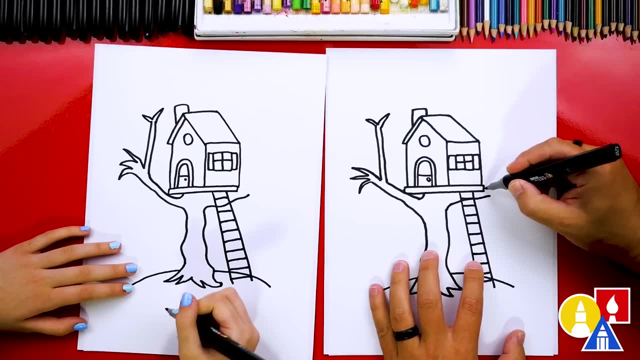 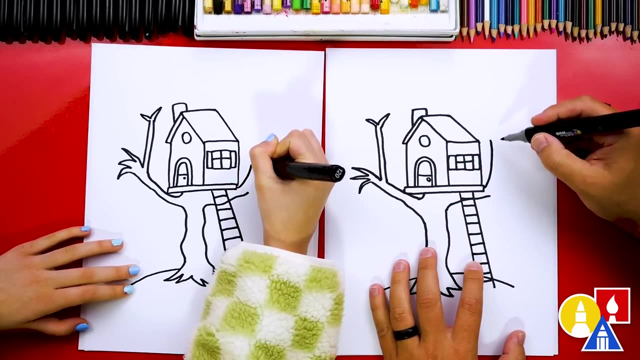 So we'll use a search from the grass up here And what he says he provides is a setup for grafting. Okay, so we're gonna draw a光 Ari flow line, Draw that and then we're done. now see if that makes sense. if i did that. 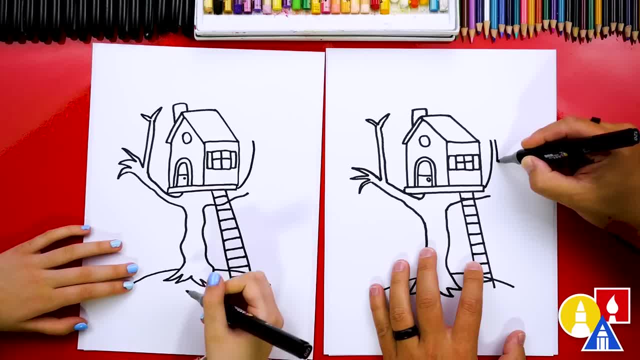 well, i did it. So i'm gonna say i'm done. Alright, let's do that, Let's leave a little space and we'll come back down. Oh, I'm going to stop there, though, And then let's draw another branch coming out this way. 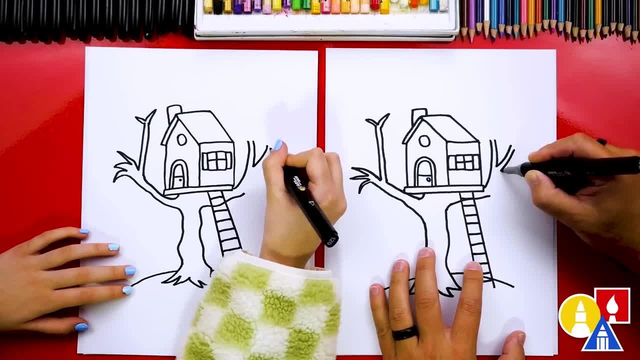 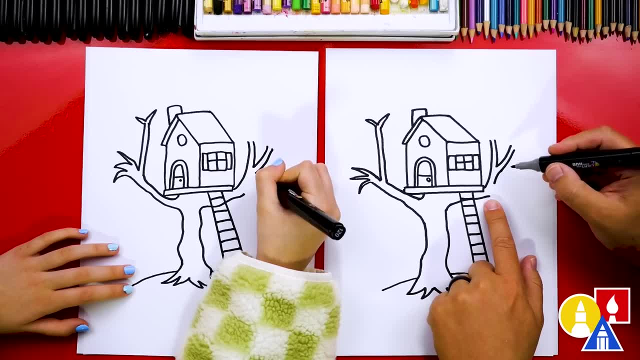 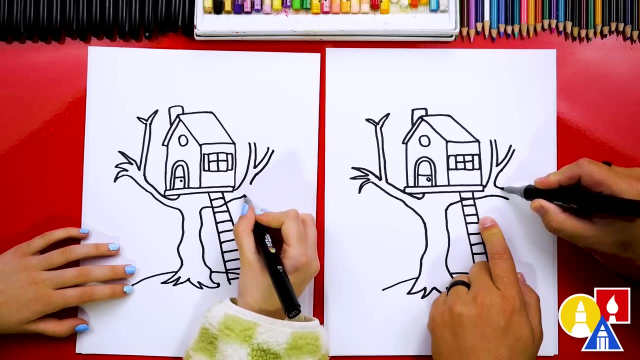 And then let's leave a little space and we'll come back down. Okay, now I'm going to curve down. So we're coming to this branch, the bigger one down here, And let's draw it curving down this way. So I'm going to draw two of these lines going this direction. 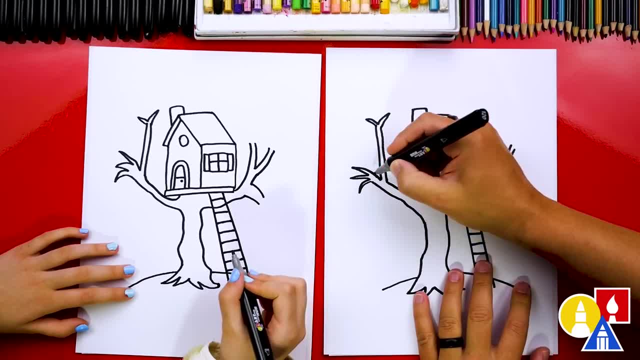 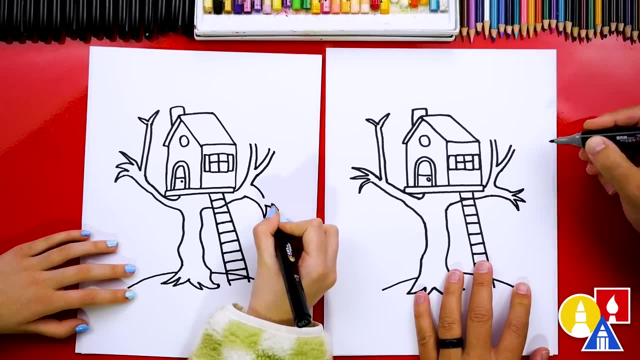 Yeah, okay, now let's draw the same kind of shape on this side. So I'm going to draw a little one, another little one and one last little branch going up, Okay, and then let's do the same thing here. 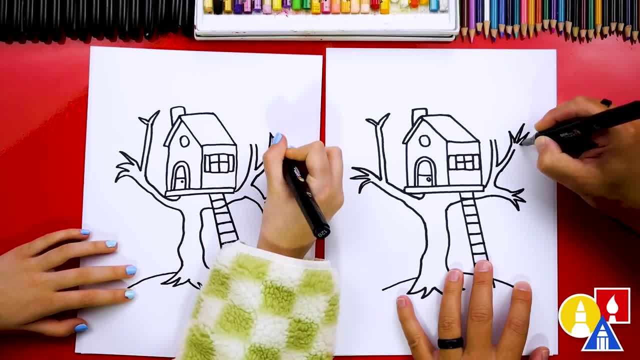 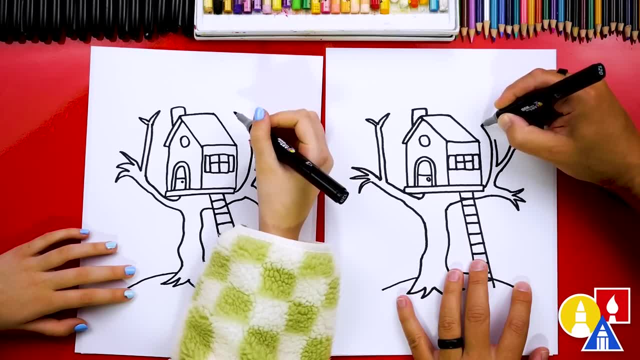 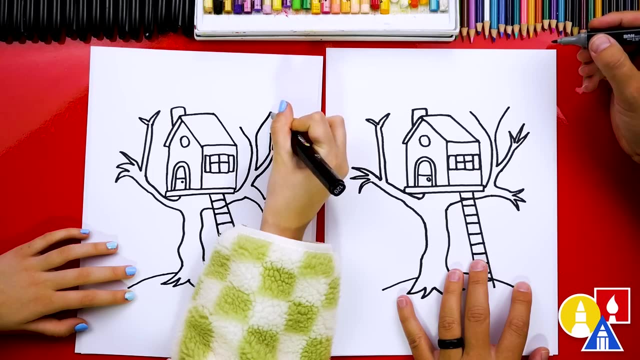 I'm going to draw three little branches that are thin and spiky coming out, And then this one- Let's draw it coming up a little higher And I'm also going to look at that. I'm going to split that branch up at the top. 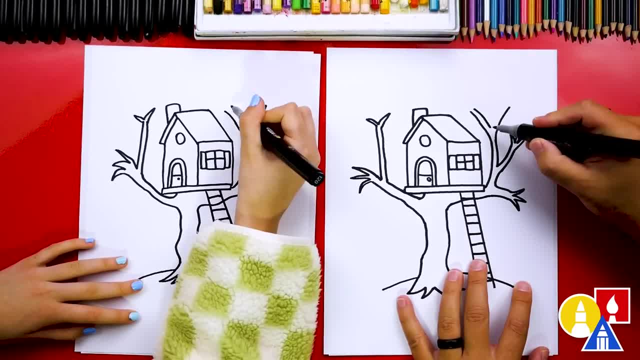 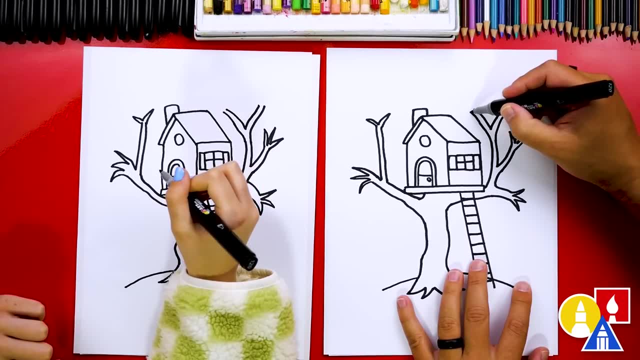 Let's leave a little space and we'll draw the letter V, coming down to the middle and back up to the other side. That's a fun way to split that branch. Okay, now let's add more spiky, smaller branches on this side. 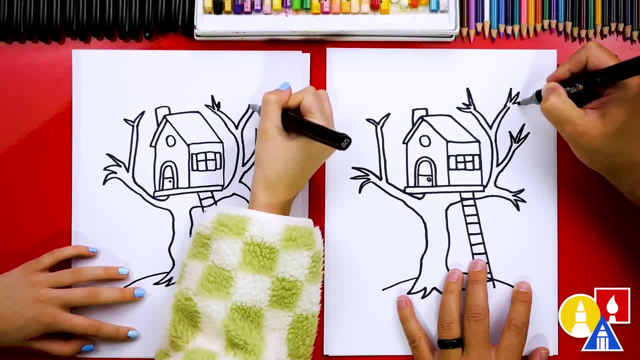 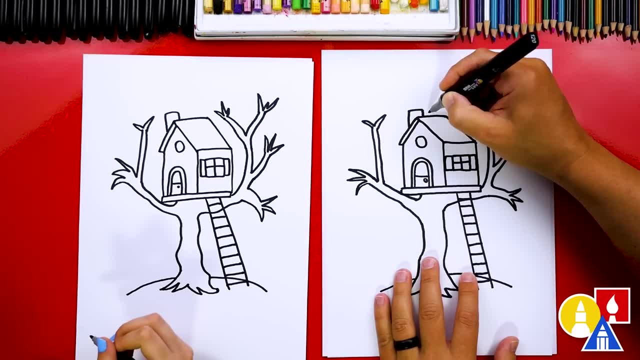 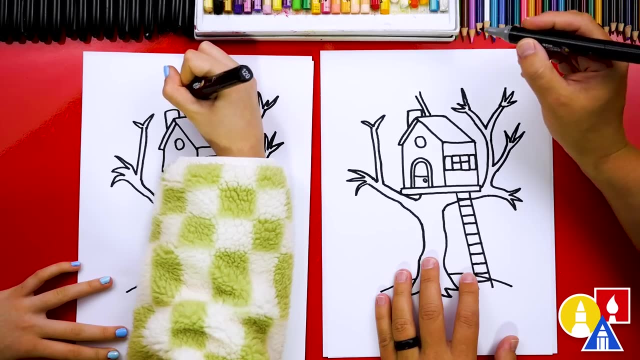 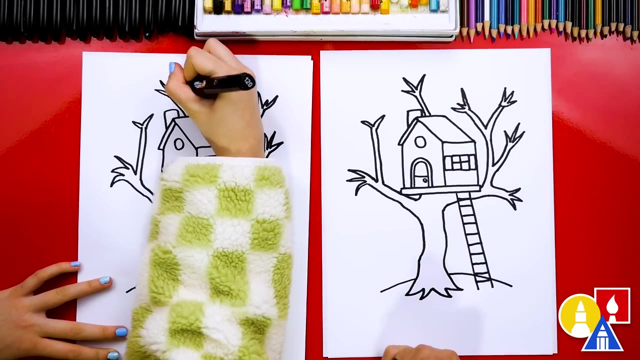 And we could do spiky, Spiky smaller branches on this side. Let's add one more branch coming out from behind our house or tree house. I'm going to draw it curving up this way And then we can draw spiky little branches on this one. 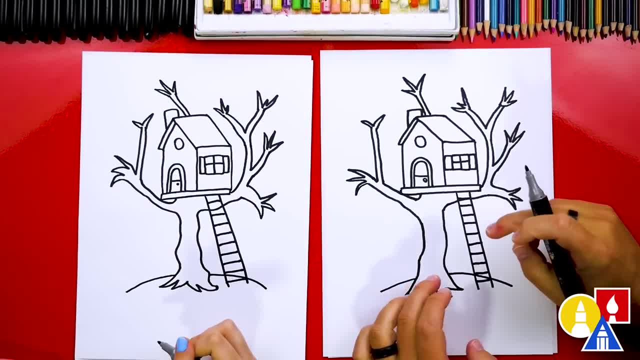 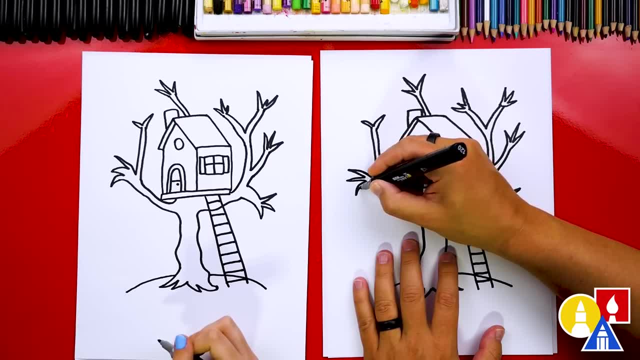 You could add even more branches, but let's leave it just like that and add the leaves, And we're just going to draw popcorn, Popcorn shapes or cloud shapes for the leaves. Let's start on this branch and I'm going to draw a bumpy line. 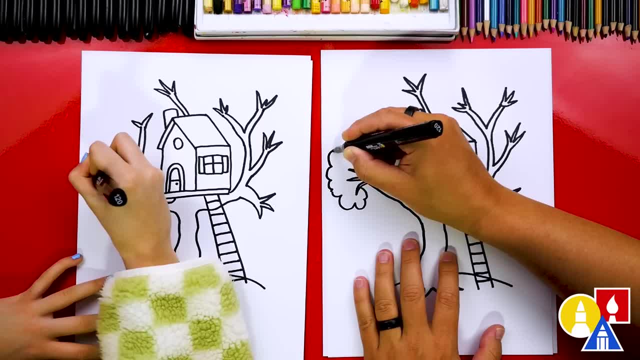 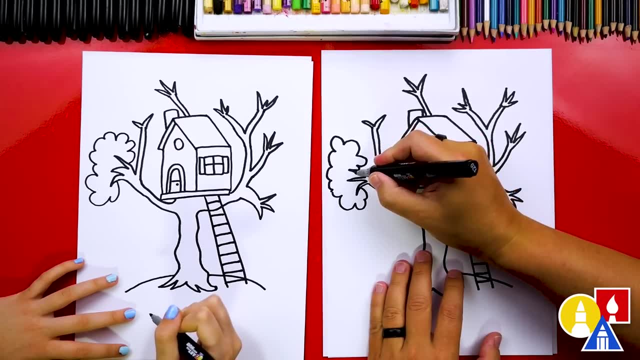 Some of the bumps are big and some are small. We're going to go all the way around until we get to the other side of the branch. Now, in between the branch we could, if we want, add two little curved lines like that: 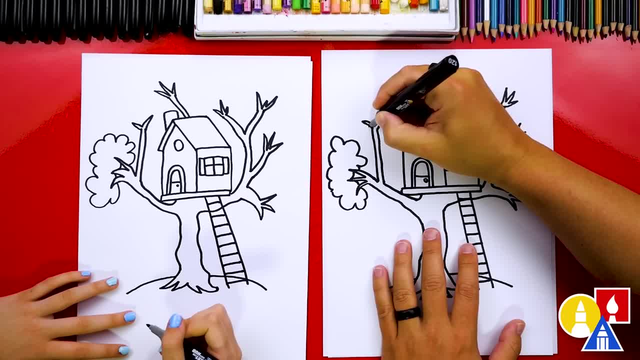 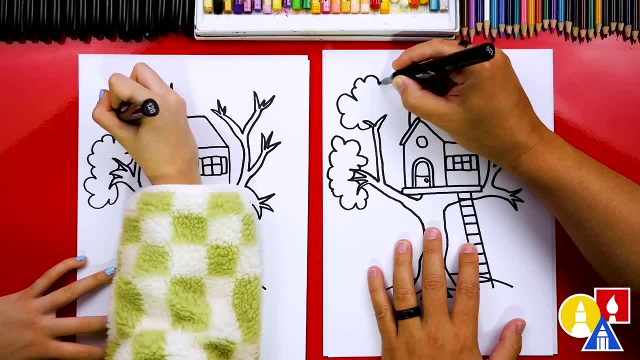 Okay, now let's add the next cloud or popcorn shape. We're going to draw it right here. I'm going to add it kind of big. Some of them are really big And then smaller. I'm going to come all the way around and down to here. 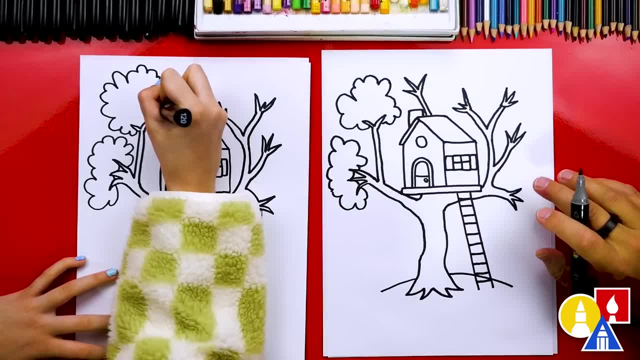 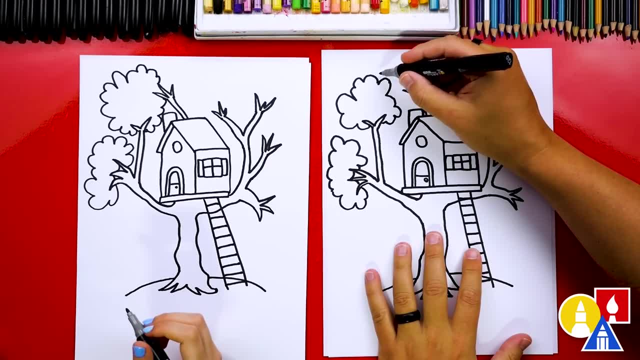 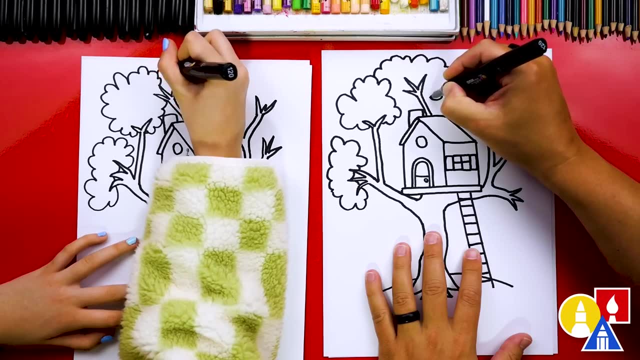 I'm still going Keep going. That's a really big shape. I like it, Thanks, Okay, Now let's add the next one right here in the middle. I'm going to start on this shape, though, and come all the way over this way. 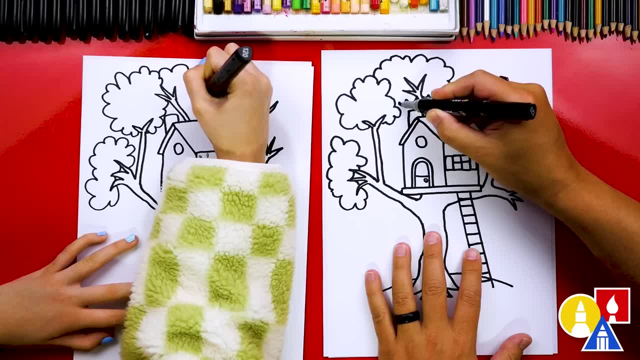 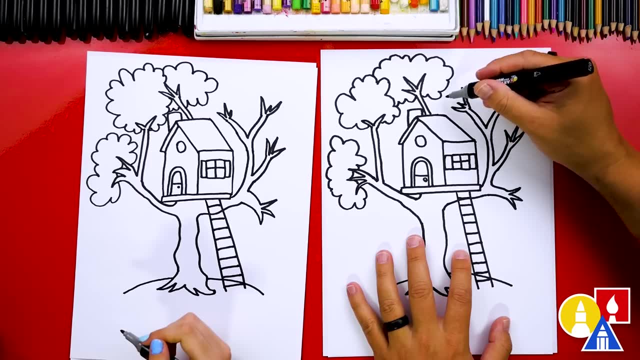 And then, right here, I connected into the branch, but then I'm going to keep going and connect to the popcorn shape here. Yeah, Okay, Now let's do the next shape, The next popcorn shape. This one will overlap behind the treehouse. 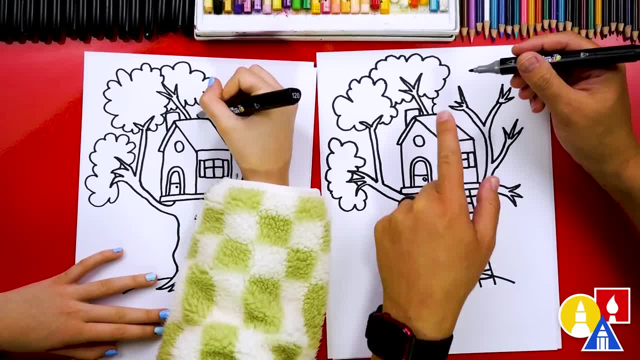 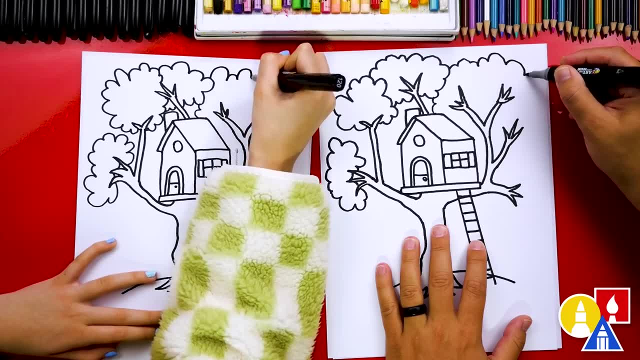 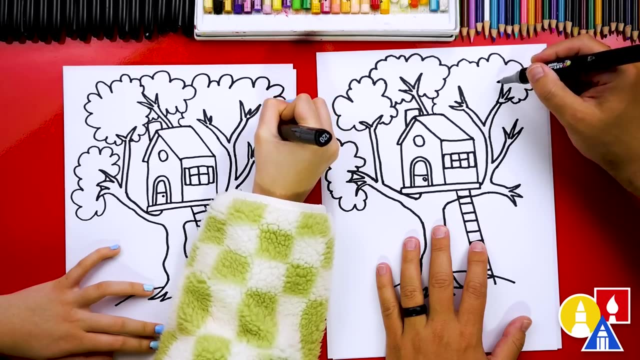 So I'm going to start here and connect to this top shape, and then we'll keep going past on the other side. Oh, maybe this one connects to the other branch here too, So I'm going to go and then stop there, And then we can also go behind the branch and then keep coming over here. 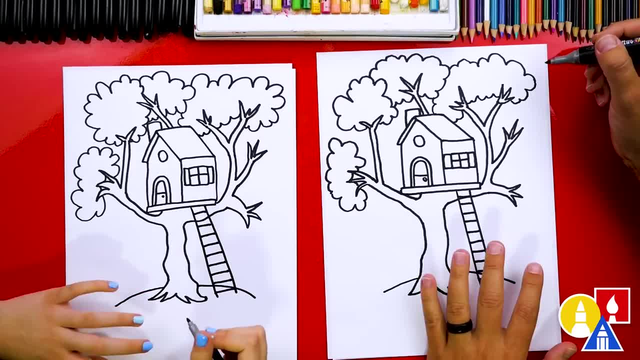 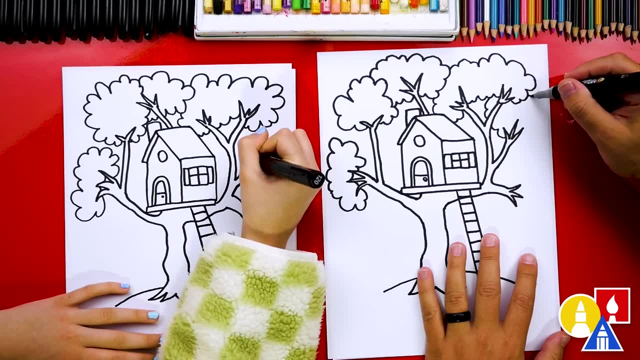 And then I'm going to go behind the treehouse again. Okay, Let's add this one next. This one will go behind this branch, And if yours is different, you can change these popcorn shapes any way you want. They don't have to look exactly like ours, right? 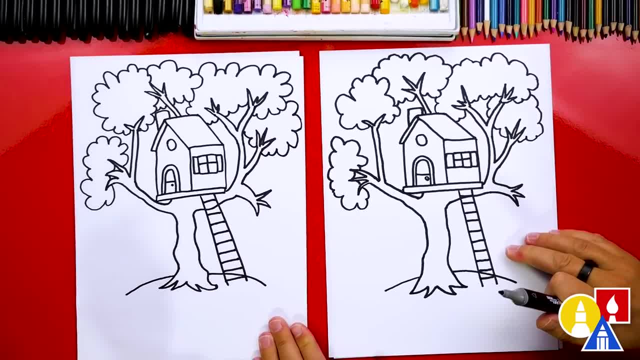 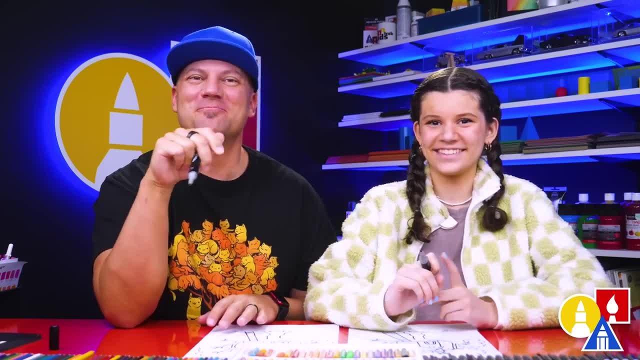 Yeah, I love that our two drawings don't look exactly the same. They're both turning out awesome, And that's because the most important thing is To have fun. Yeah, To have fun And also To practice, Practice. Remember to have fun and practice. 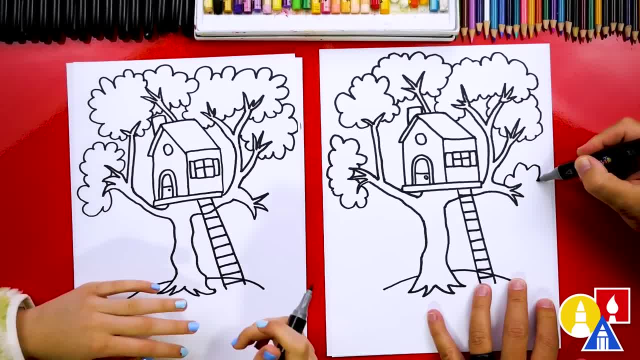 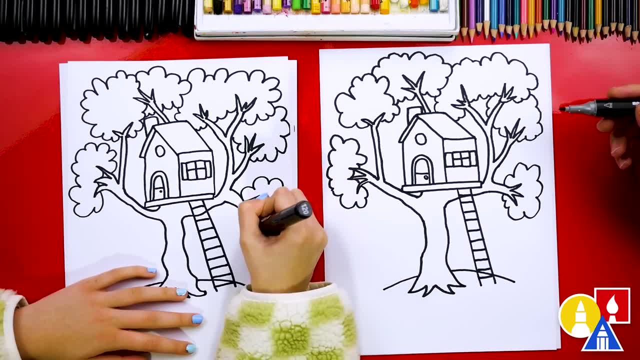 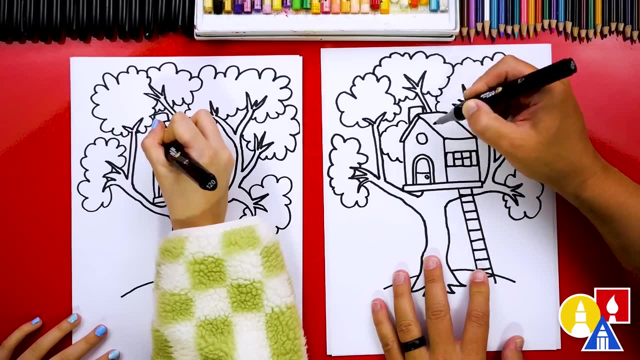 Okay, Let's keep going. We're almost done. Let's add another shape right here on the last branch. We're going to draw it coming around and connecting to the other side. Oh, I even want to add one more little group of leaves right here behind the treehouse. 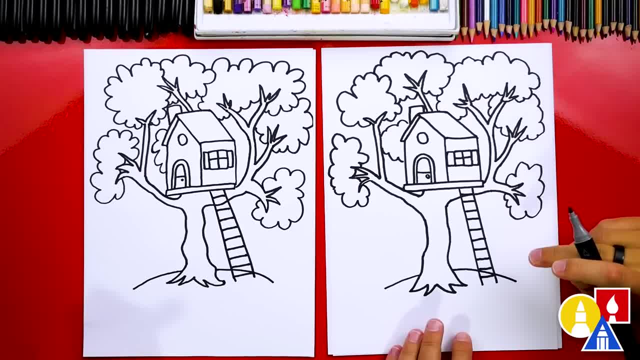 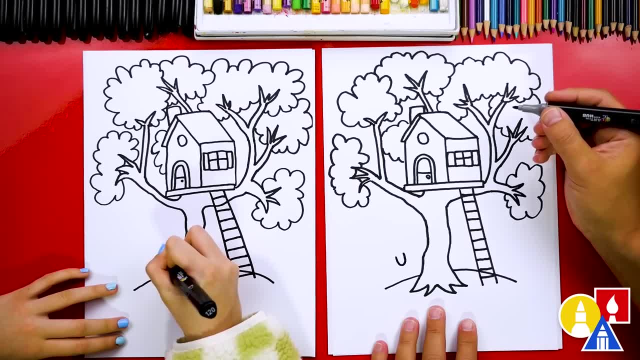 We did it. We finished our tree. Let's add a couple more things to make it look more like spring. Let's draw some tulip flowers right here. I'll draw a U shape And then we can draw a diagonal line inside and a shorter diagonal line going the other way. 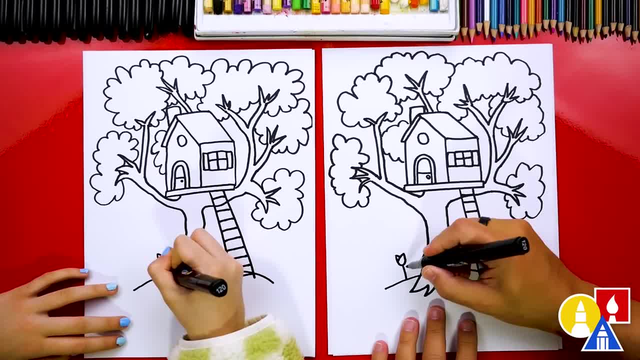 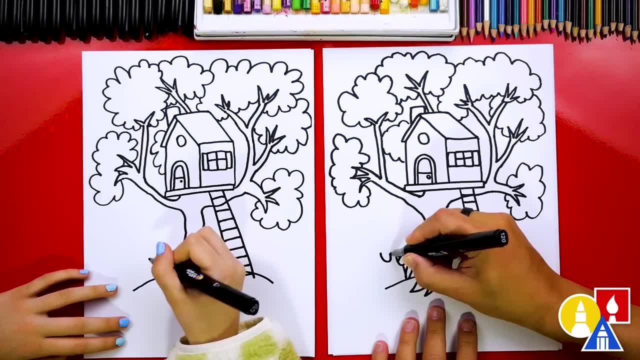 Then we could draw the stem And we can also draw a leaf. We'll come out and then back down. Let's repeat that a couple more times to add more tulips. We're just going to use those same steps. I went a lot faster. 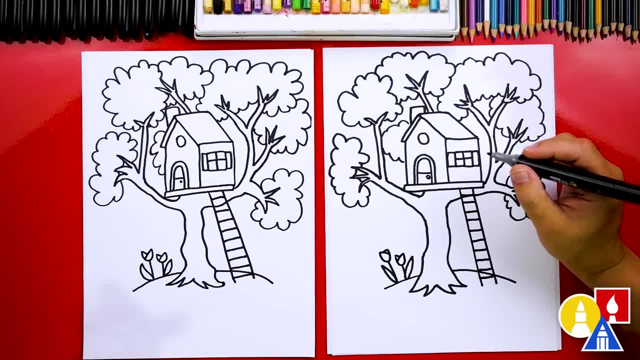 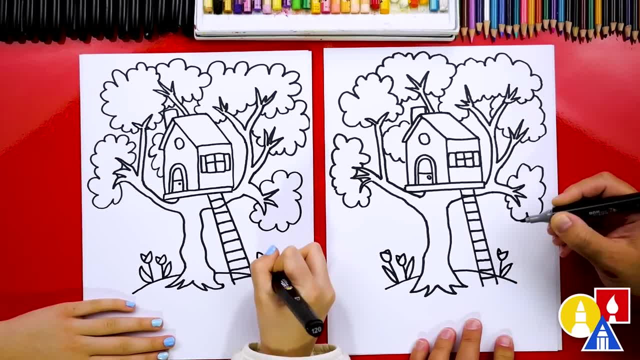 So remember, you can pause the video if you need extra time. Oh, let's add even more flowers on this side, And you can even add different flowers. Oh, let's just draw a simple daisy. I'll draw a circle in the middle. 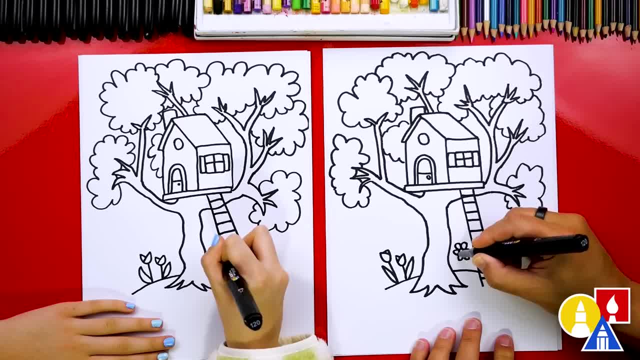 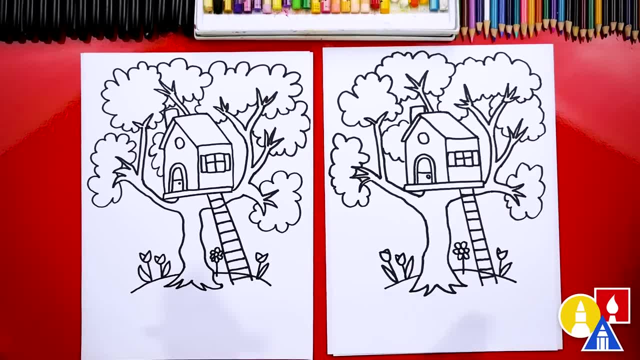 And then we'll draw the petals that go all the way around, And then a stem down. We could draw a lot more flowers. Yeah, Let's leave it just like this, But we're not completely done. We still need to color it. 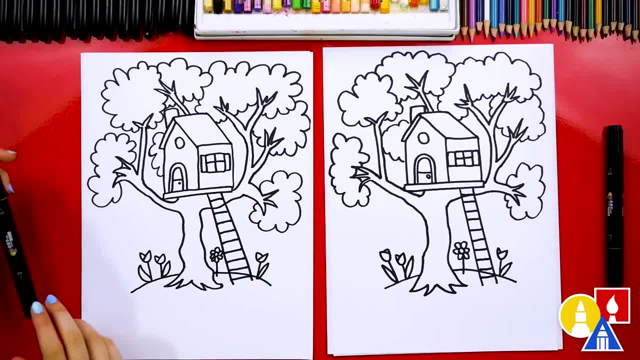 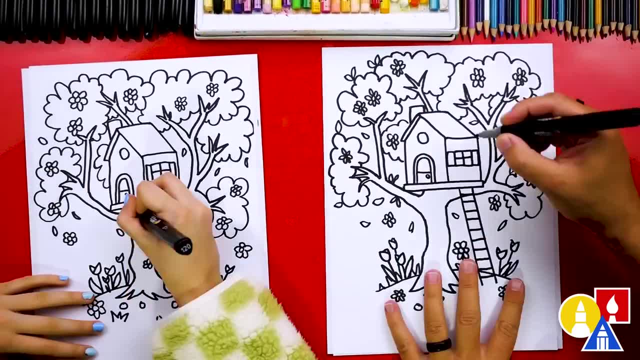 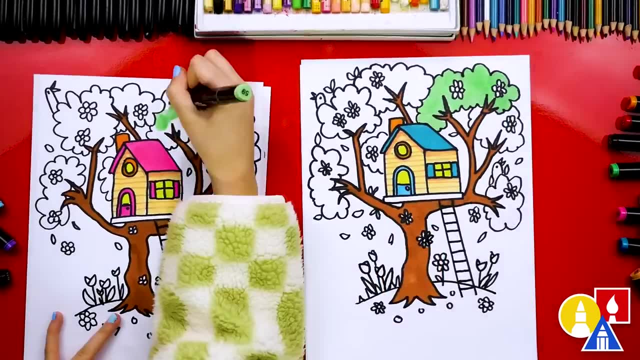 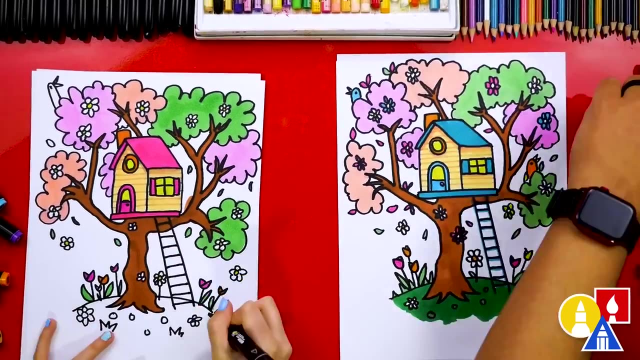 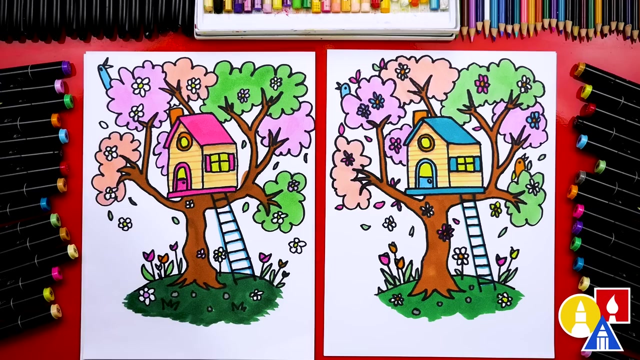 Yes, We are going to fast forward, So remember to pause the video and take time to color your drawings. You ready to speed things up? Yeah, Let's go. We did it. We finished drawing and coloring our spring treehouse. It looks so much better colored in. 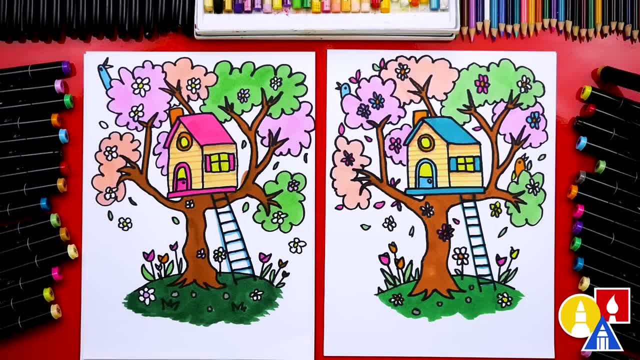 Yeah, We used our markers to color with. If you have the same Art For Kids Hub set, you can use the same colors that we used. But also remember, you don't have to. You can use a different brand of markers or even crayons or colored pencils. 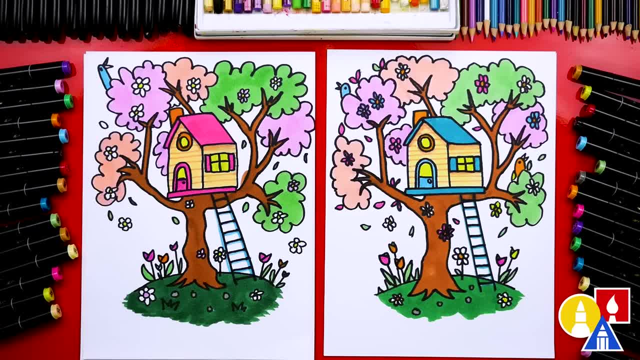 Now, if you do have the same set, we used 103 Brown for the tree. 156 is the darker green we used for the grass. Then we used two different pinks. We used a dark pink, 88. And a light pink.